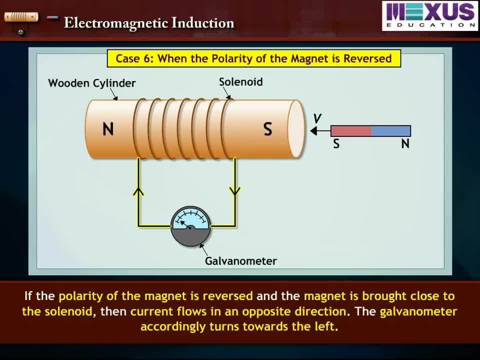 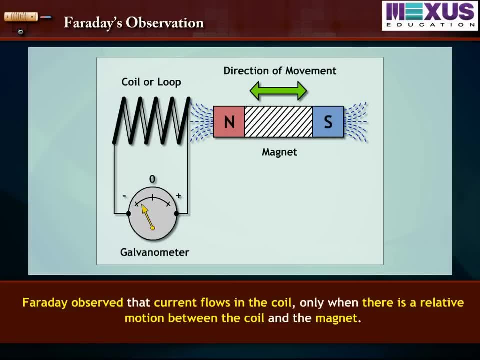 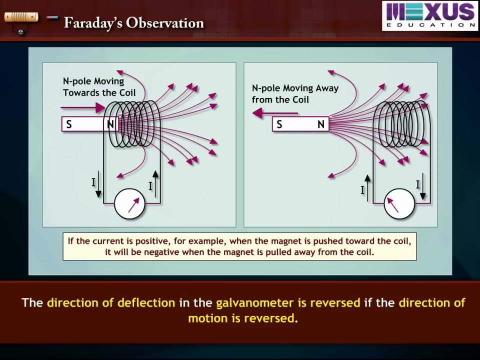 then current flows in an opposite direction, The galvanometer accordingly turns towards the left. Faraday observed that current flows in the coil only when there is a relative motion between the coil and the magnet Capacities of depth of current. The direction of deflection in the galvanometer is reversed. if the direction of motion is reversed, 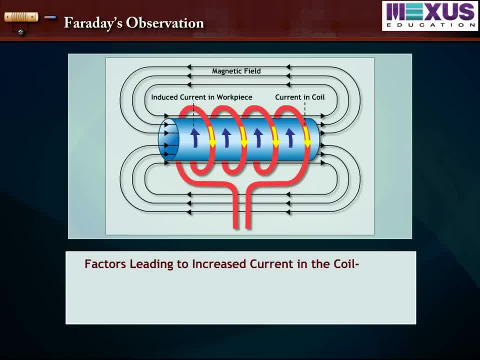 Un souha potable. The current in the coil and the corresponding deflection of the galvanometer can be increased by using a strong magnet or or by increasing the motion of the magnet. Increasing the area or the number of turns also creates a strong current in the coil. 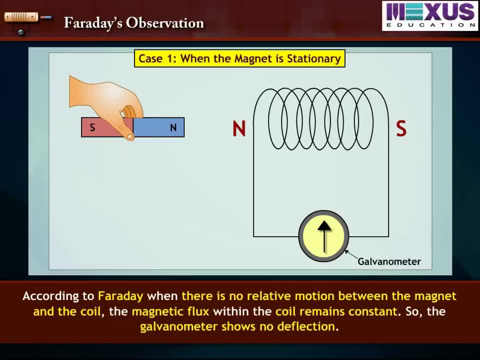 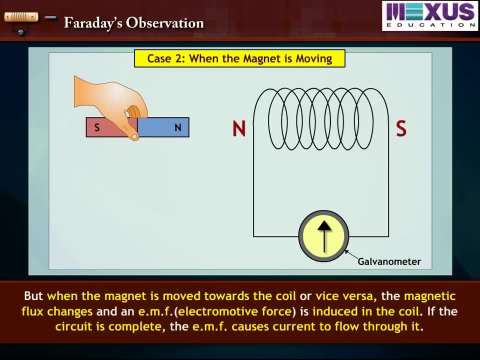 According to Faraday, when there is no relative motion between the magnet and the coil, the magnetic flux within the coil remains constant, So the galvanometer shows no deflection. But when the magnet is moved towards the coil or vice versa, the magnetic flux changes and an EMF is induced in the coil. 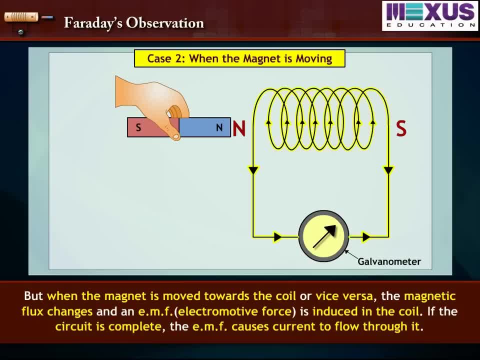 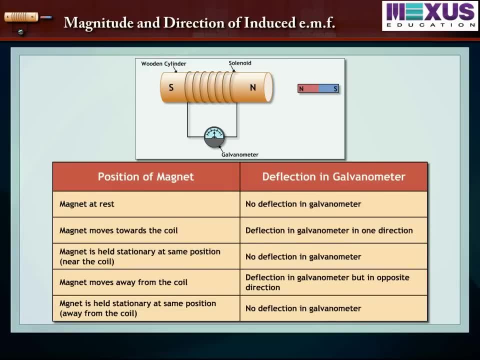 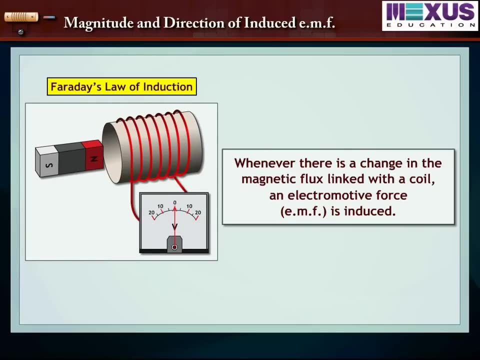 If the circuit is complete, the EMF causes current to flow through it. Based on his experiment, Faraday formulated two laws of electromagnetic induction. Whenever there is a change in the magnetic flux linked with the coil, an electromotive force is induced. 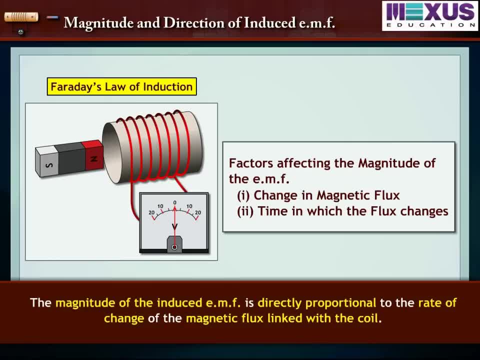 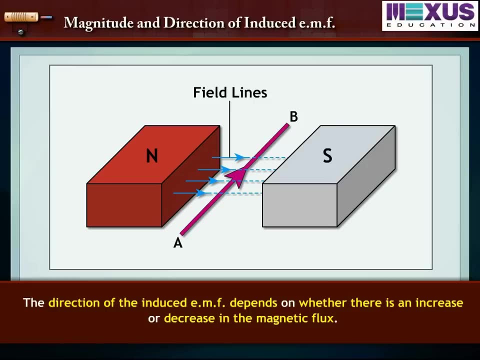 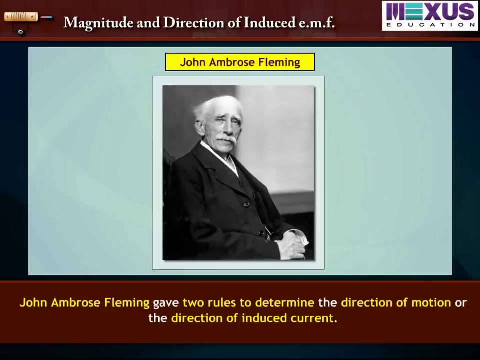 The magnitude of the induced EMF is directly proportional to the rate of change of the magnetic flux linked with the coil. The direction of the induced EMF depends on whether there is an increase or decrease in the magnetic flux. John Ambrose Fleming gave two rules to determine the direction of motion. 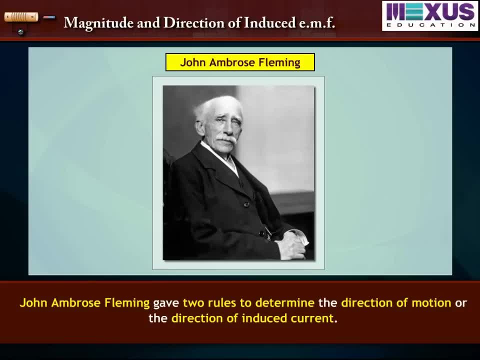 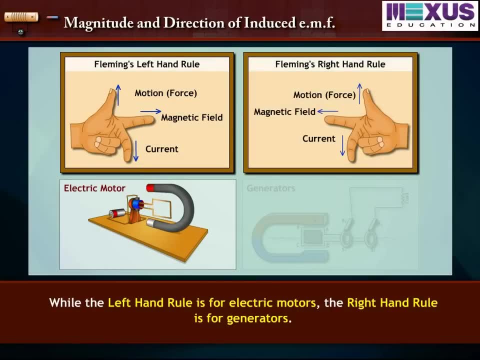 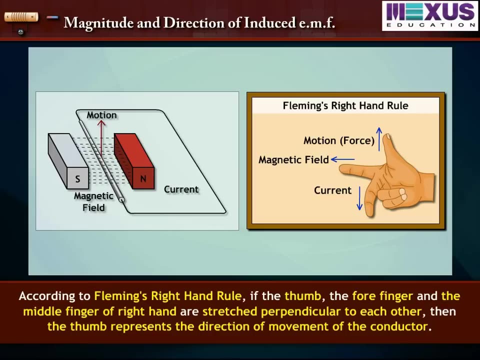 or the direction of induced current. While the left-hand rule is for electric motors, the right-hand rule is for generators. According to Fleming's right-hand rule, the thumb, forefinger and middle finger of right hand are stretched perpendicular to each other. 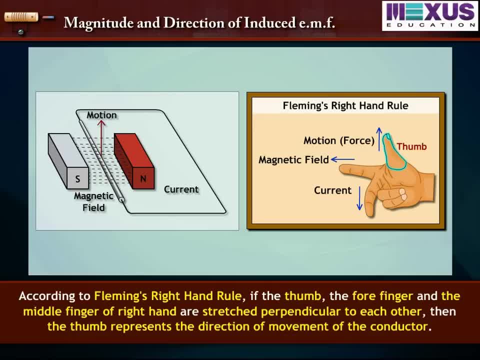 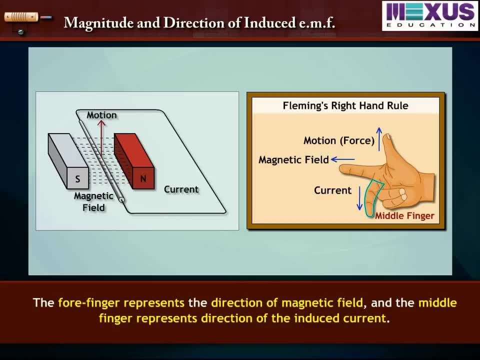 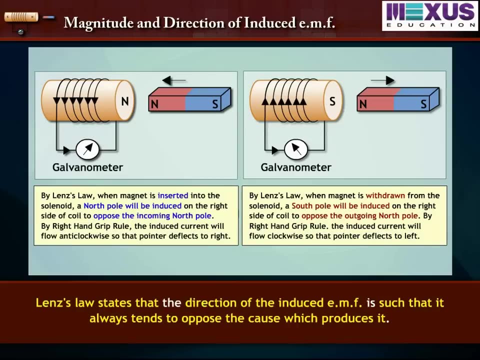 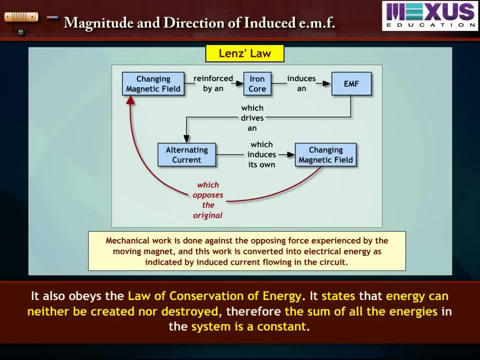 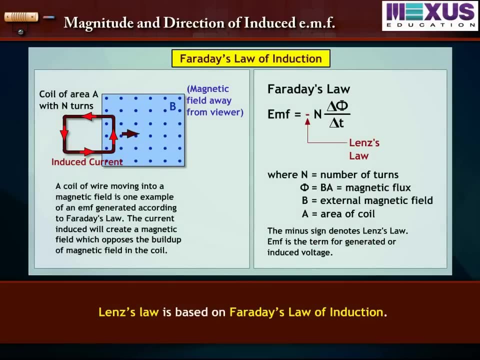 It also obeys the law of conservation of energy, It stating that energy can neither be created nor destroyed. Therefore, the sum of all the energies in the system is a constant. Lenz's law is based on Faraday's law of induction. Lenz's law is based on Faraday's law of induction. 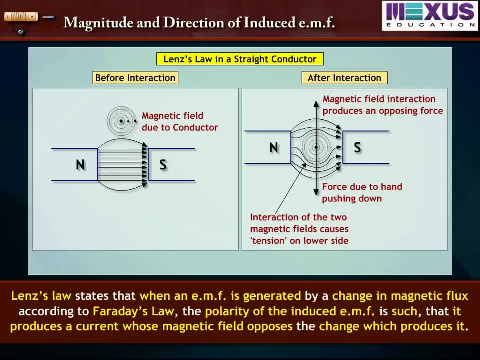 Lenz's law states that when an EMF is generated by a change in magnetic flux according to Aspen analysis, Lenz's law states that when an EMF is generated by a change in magnetic flux according to Aspen analysis, According to Faraday's law, the polarity of the induced EMF is such that it produces a current whose magnetic field opposes the change which produces it. Thank you for watching.